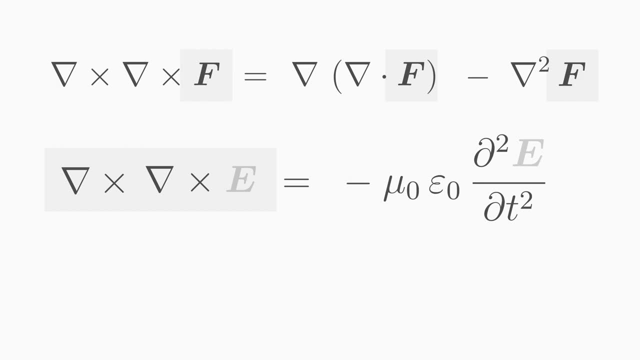 minus the divergence of the gradient of F. This is just a relationship that can be derived. In our case, F is the electric field, E, So let's substitute the double cross product with this relation. The first Maxwell equation tells us what the divergence of the electric field is. 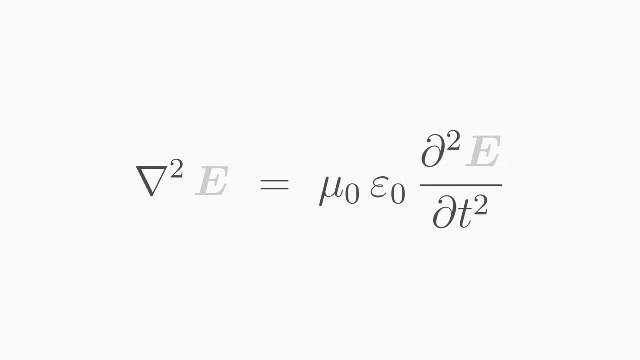 It is zero, So we can omit this term. So we can omit this term. The derivative of the wave equation for the electric field E in vacuum. The derivative of the wave equation for the B-field is analogous. You get exactly the same wave equation, only that instead of the letter E, 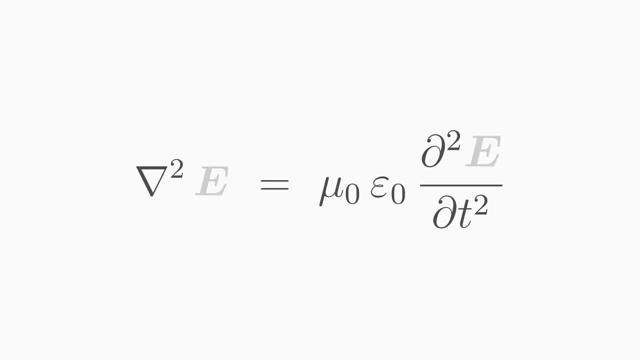 you get the letter B in the wave equation. How do we know that we now have a wave equation? Well, by comparing our result with a general form of a wave equation. Here VP is the phase velocity of the wave. It indicates how fast a wave crest of the wave propagates from A to B. If you compare the two wave equations, 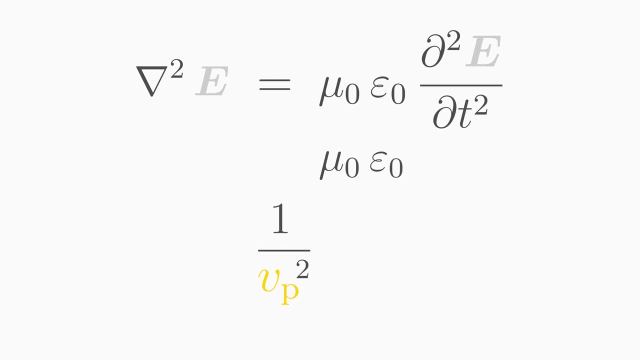 you see that µ0 times ε0 must be equal to 1 divided by vp squared Rearrange for the phase velocity. Both µ0 and ε0 are physical constants whose values we know. If you insert values for the physical constants then you get a certain value for the phase velocity of the electric wave. 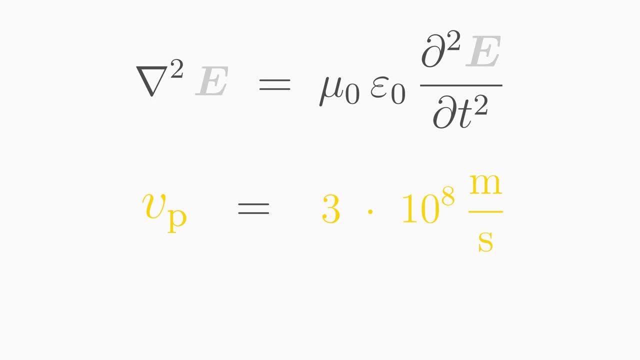 E. This value should be familiar to you. As you can see, the solution of the wave equations for E-field and B-field propagate with the speed of light c. We can express our derived wave equation with the speed of light c. Let's briefly look at the structure of the wave equation. 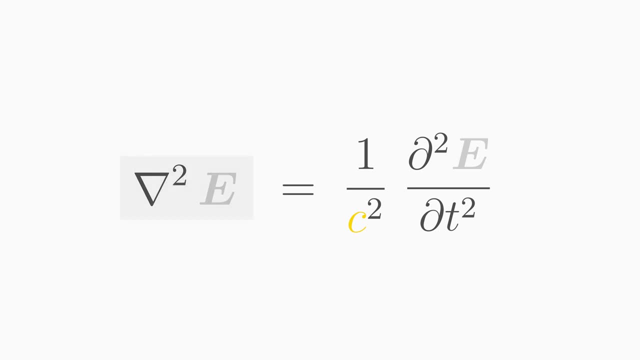 On the left side of the wave equation is the space change of the wave and on the right side is the temporal change. This wave equation is a vector field equation for the E-field and represents a very compact notation for three scalar wave equations. µ0²E is, in the three-dimensional case, a vector with three components. 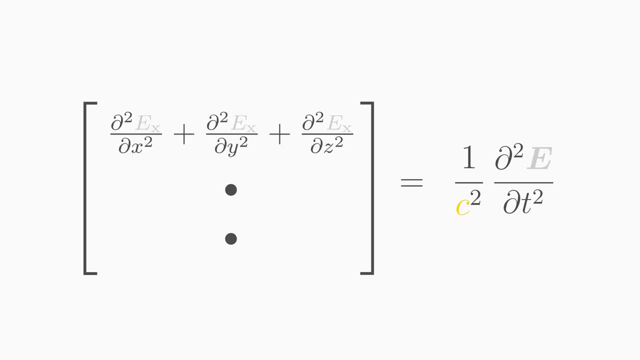 If you write out this vector, you get, for the first component, the sum of the second derivatives of EX, with the same value. If you write out the sum of the second derivatives of EX, you get, for the second component, the sum of the second derivatives of EX, with the same value. 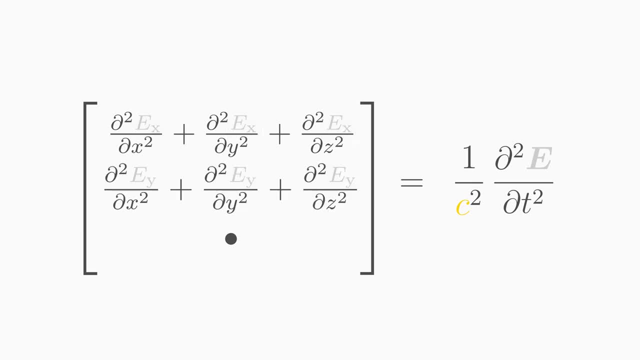 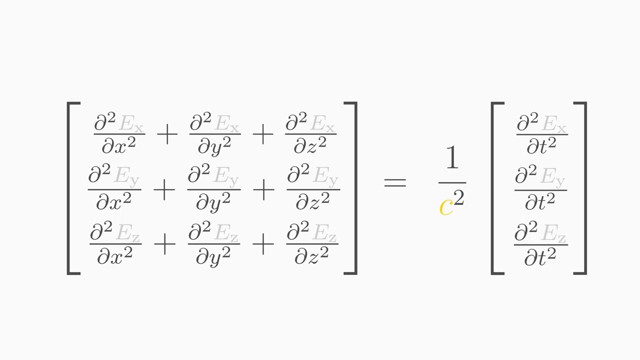 respect to x, y and z. For the second components you get the sum of the second derivatives of e- y and for the third component, the sum of the second derivatives of e z. The right hand side is a vector containing the time derivatives of the e-field components. These are three non-coupled 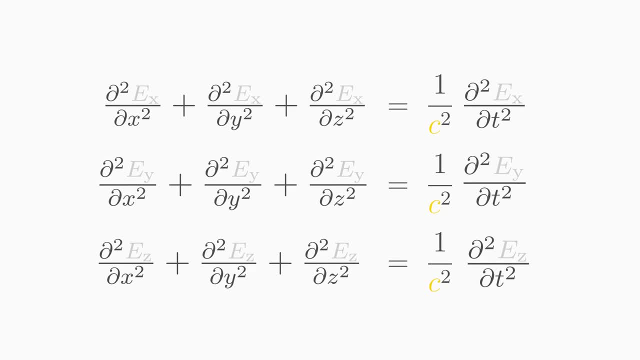 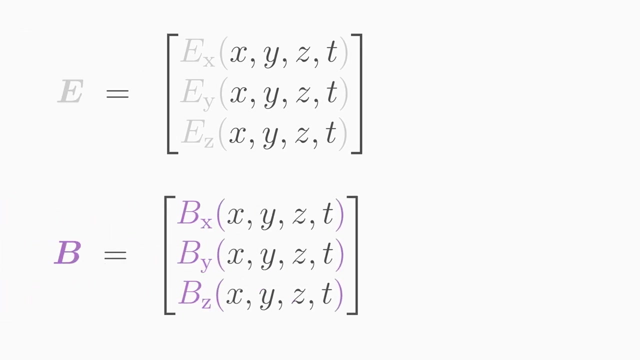 partial differential equations of second order. Their solution gives the e-field of the wave at any time and at any location. If you solve the first differential equation, then you find out how the first e-field component changes in time and space, With all three components of the e-field and the three components of the b-field. 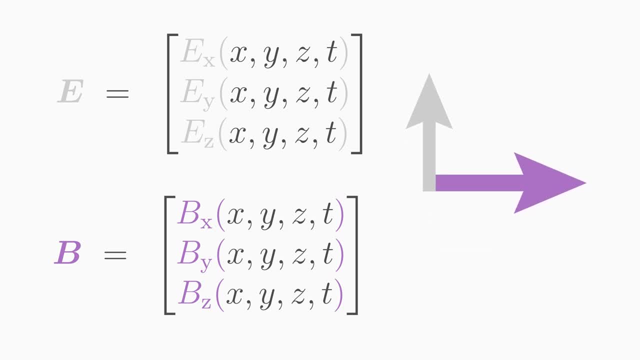 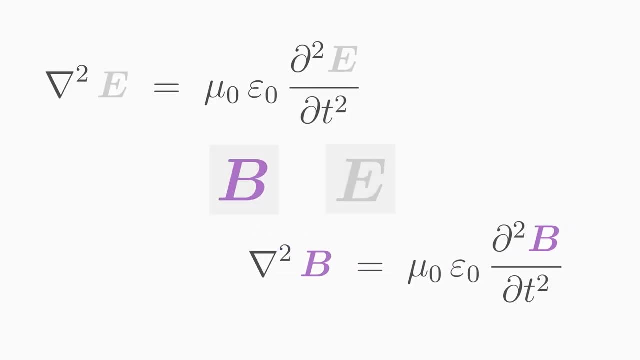 you know the entire temporal and spatial behavior of the electromagnetic wave Solution of the wave equation is a wave, but not necessarily an electromagnetic wave. The solution of the wave equation must also fulfill all Maxwell's equations in vacuum. Let's see what other conditions the solution of the wave equation for b and e-field must satisfy. 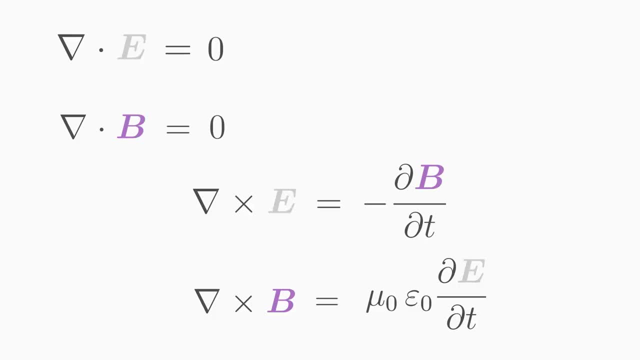 to be an electromagnetic wave. To see what condition is required by the first Maxwell equation, let us consider as an example a specific solution of the wave equation, namely a three dimensional plane wave described by the first Maxwell equation. E0 is a vector pointing in the direction of e and has three amplitudes in x, y and z direction. as 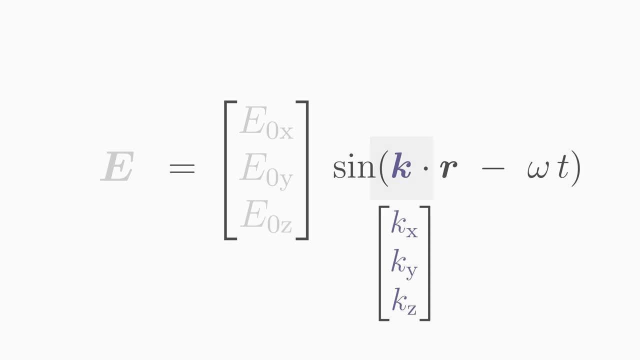 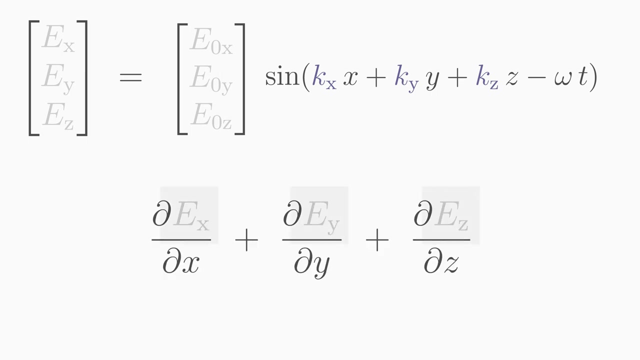 components. k is the wave vector and defines the direction of propagation of the wave. Omega is the angular frequency of the wave. You can also write out the scalar product of k with the position vector r like this: The divergence of the e-field is the sum of the derivatives of the individual field components. 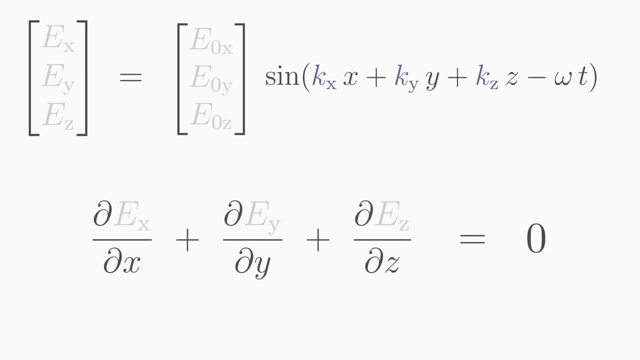 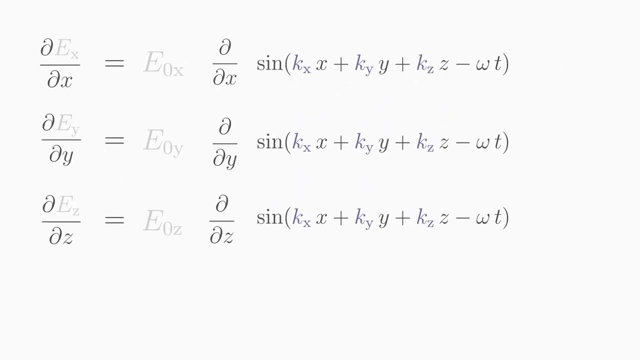 with respect to x, y and z, And this sum is supposed to be zero according to Maxwell's equation. Let's calculate the derivatives. The derivative of sine with respect to x is cosine and the wave number kx is added as a factor in front of it. 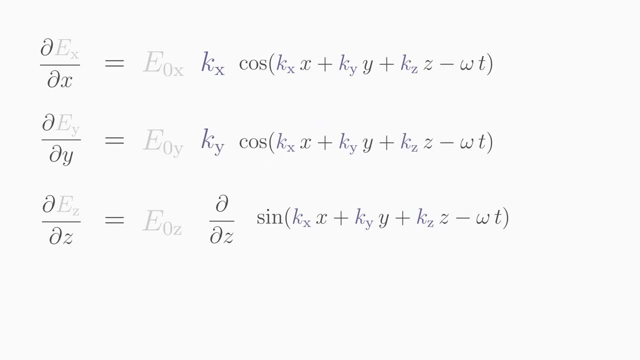 Then we have the derivative of sine with respect to x and the wave number kx is added as a factor in front of it. Then we differentiate the sign with respect to y and then with respect to z, We can factor out the cosine. The sum in the parentheses corresponds exactly to the scalar product between the wave vector. 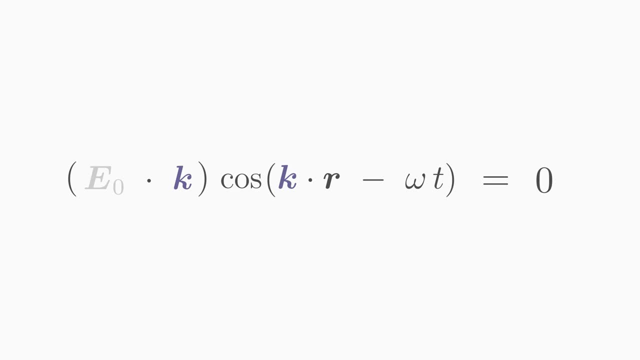 k and the E-field vector, with the amplitudes For the first Maxwell equation to be zero for all times, t and locations x, y, z, the scalar product must be zero because cosine function is not always zero. of course. For the scalar product to be zero, the wave vector and the E-field vector must be orthogonal. 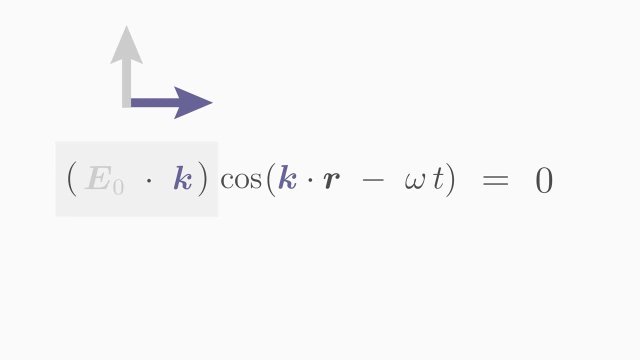 to each other at all times and locations. Thus Maxwell's first equation in vacuum requires that the E-field oscillates only perpendicular to the direction of propagation. If you take a plane wave for the B-field and proceed analogously with the second wave, 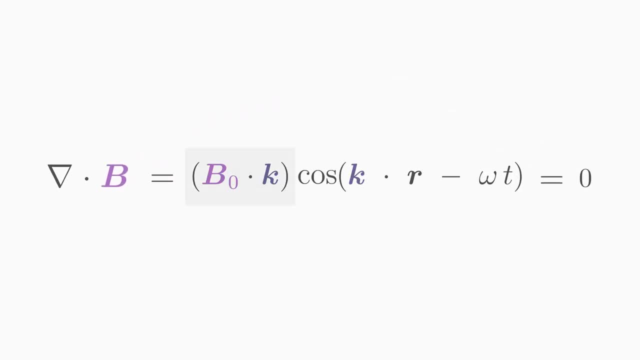 then you will find out that also the B-field is always orthogonal to the direction of propagation. Let us take the fourth Maxwell equation for the curl of the B-field. We know from mathematics that the resulting vector of the cross product is always orthogonal to the vectors between which the cross product is formed. 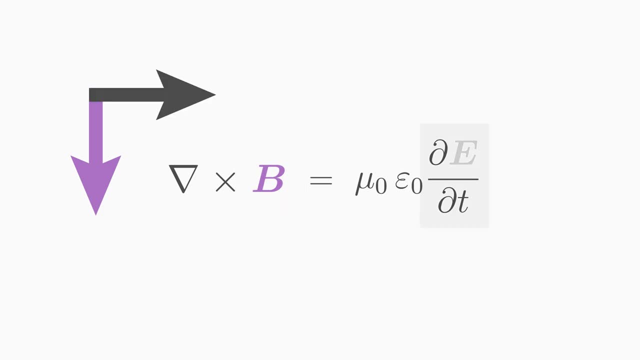 So in this case the B-field vector is orthogonal to the vector that is the derivative of the E-field. In the case of a plane wave, the E-field vector and its time derivative point in the same direction. Thus the B-field is not only orthogonal to the derivative of the E-field but also to 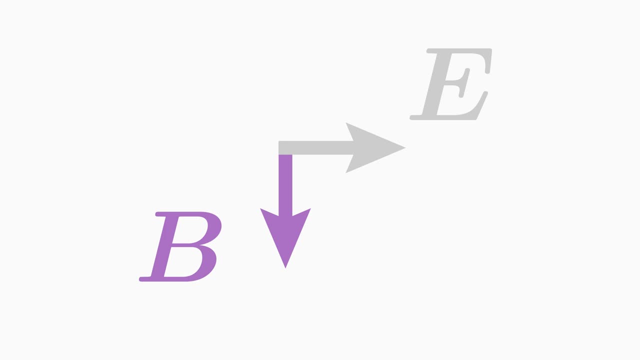 the E-field vector itself. The same condition is also required by the third Maxwell equation. The E-field of an electromagnetic wave in vacuum must always be orthogonal to its B-field. So we can summarize An electromagnetic wave propagating in vacuum with speed of light as a B-field and E-field. 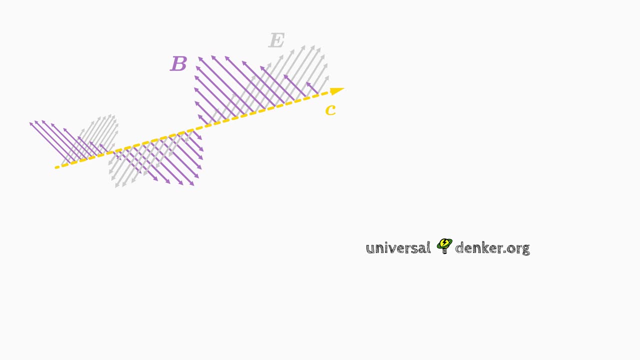 The two field vectors are always orthogonal to each other and to the direction of propagation of the wave. With this in mind, bye and see you next time.